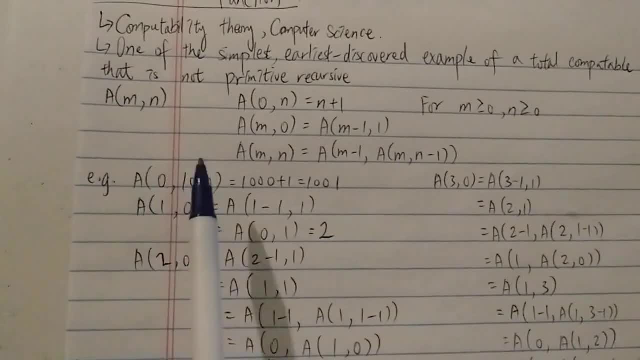 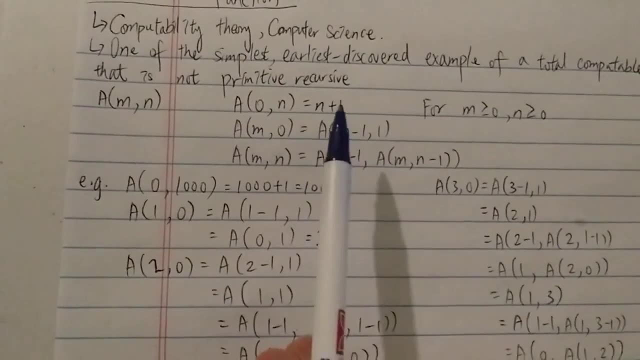 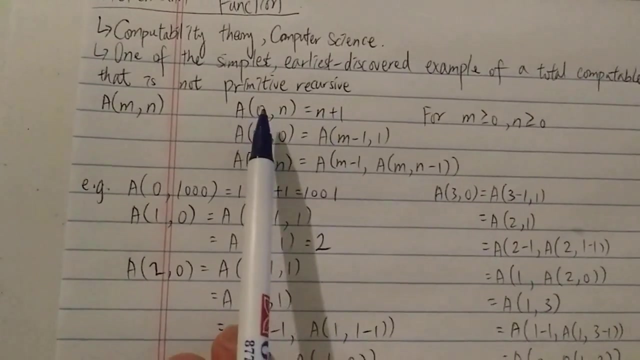 thing about this computer function. so first, the first example is a 0, 1,000. so we're gonna look at the first argument first. like I said, the first argument is quite straightforward. so is a 0 of 1,000. it just equal to, of course, the first. 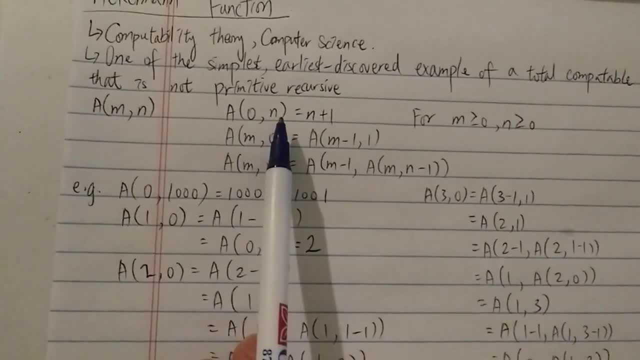 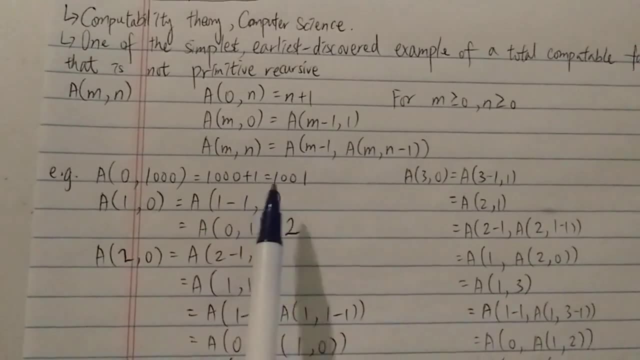 argument sets: and if M is 0 and you just equal to n plus 1, so a of 0, 1,000 it just equals to 1,000 plus 1, which is 1,001. of course you can put a Google here and the. 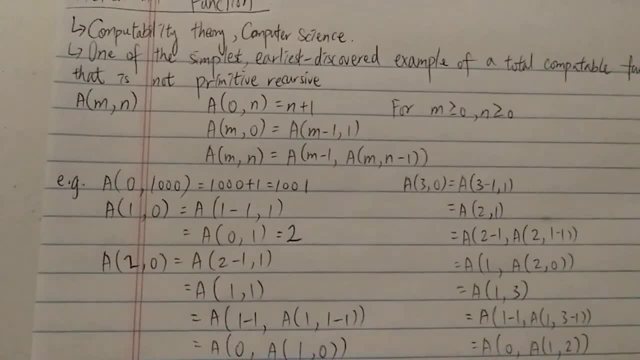 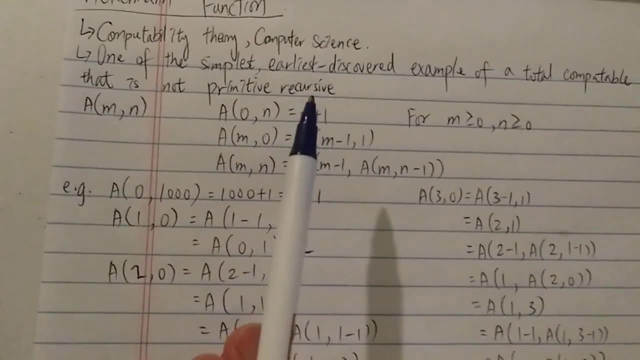 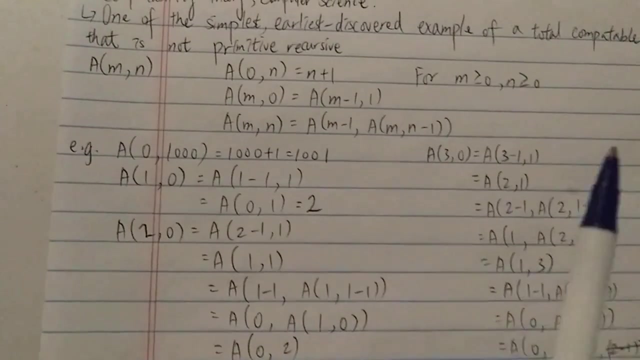 answer would be Google plus 1. so, as long as you can already see, as long as M is 0 or very, very small, like you know, then you won't get a very big result, and in the second example we're gonna start looking at the second argument. so let's. 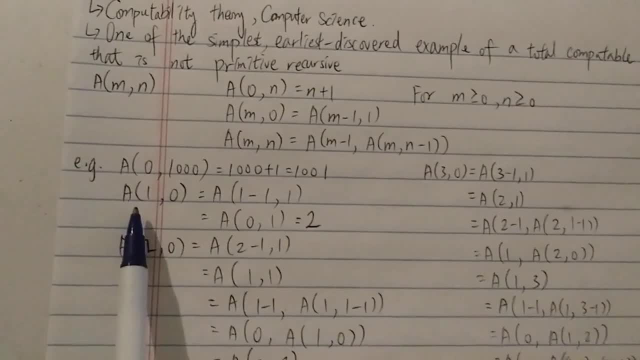 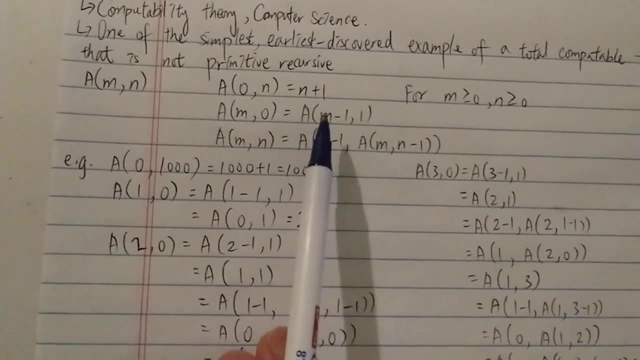 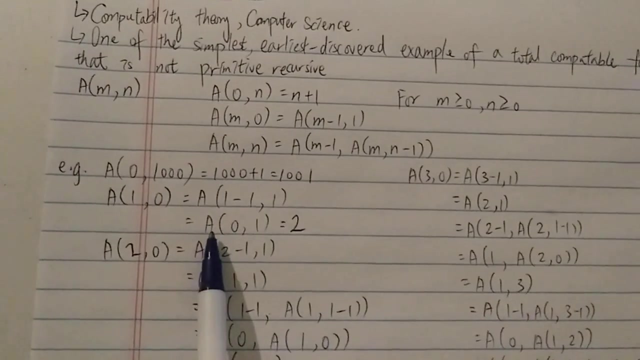 start, it start with a very small number, 1. so again you can only put positive integers here. so a 1, 0 is equal to a. of course you're looking at the second one and then it becomes a 0- 1, because 1 minus 1 is 0, and then it equals to 2. 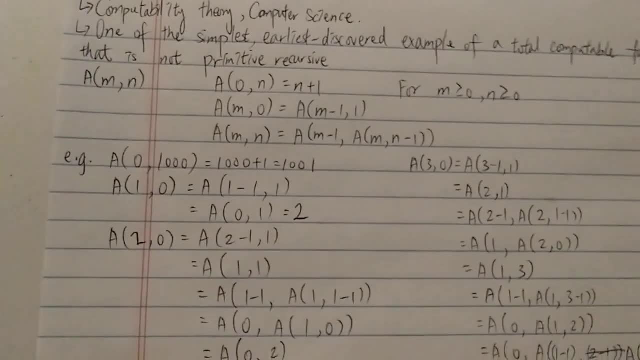 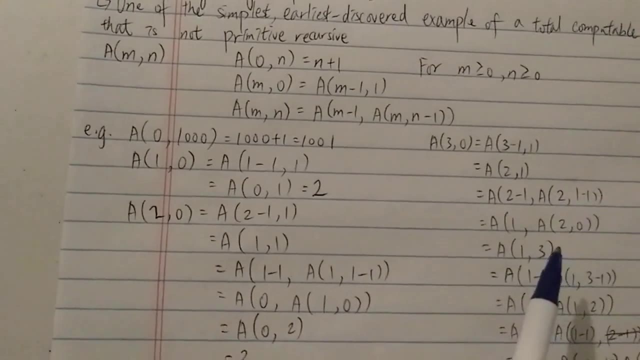 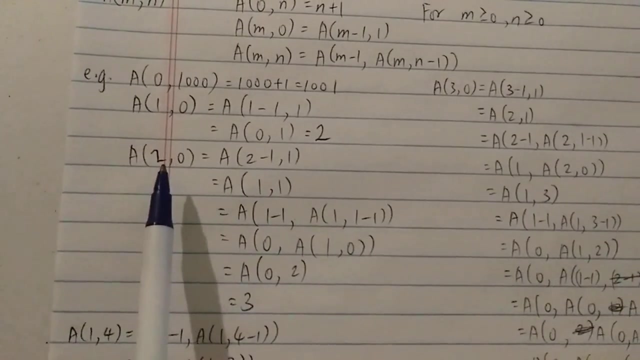 which is the first argument. n plus 1 is a, 1 plus 1 is 2. so, of course, 1: 0 is still kinda straightforward, because they are so such a small number. however, let's look at another. you know, relatively it looks simple. but let's look at a 2, 0. so 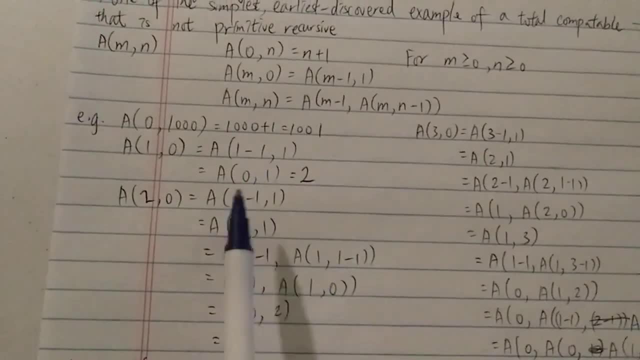 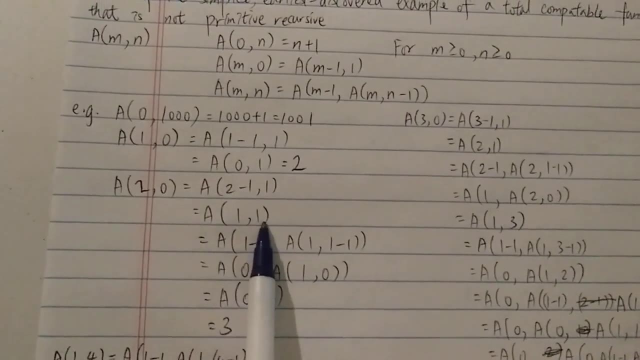 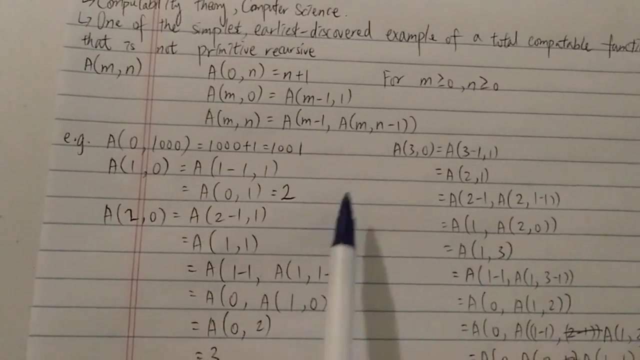 a 0 is equal to, of course. you look at the second argument, so it becomes a 2 minus 1, 1, and then it becomes a 1 of 1, and then, of course again, since both M and n is not 0, you have to look at the third argument over here, so it becomes a. 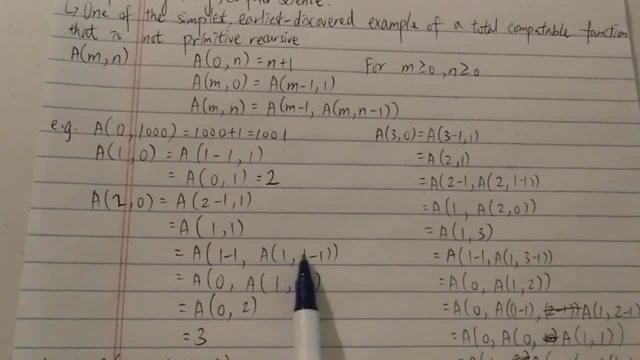 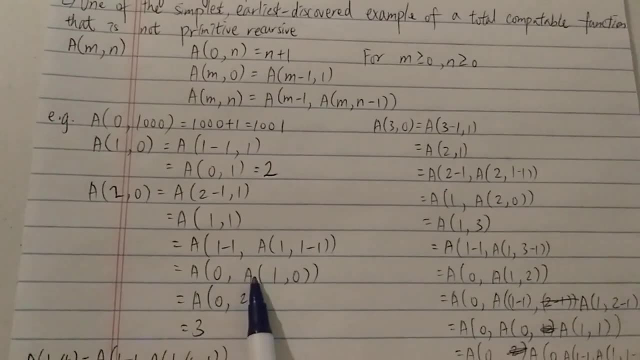 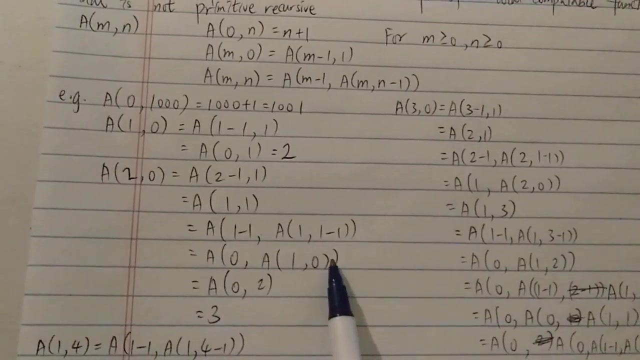 of 1 minus 1 and then a of 1- 1 minus 1, because you're looking at the third argument- and then it becomes a of 0 and then a of 1 minus 1 and then a of 1, 1 a 1- 0. so here it becomes straightforward again, because you finally get some 0. 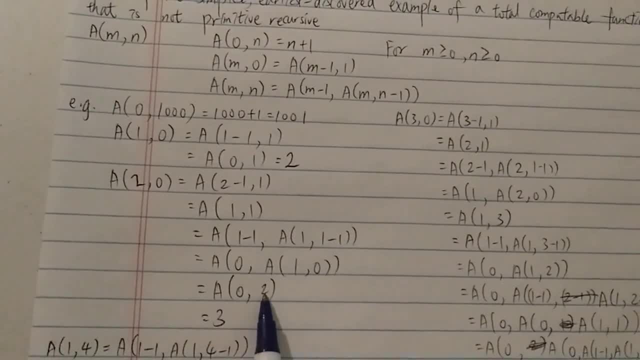 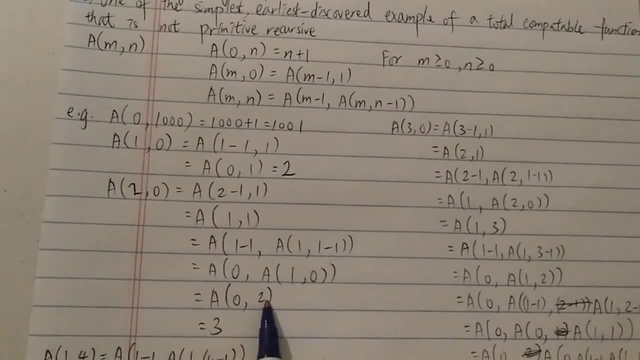 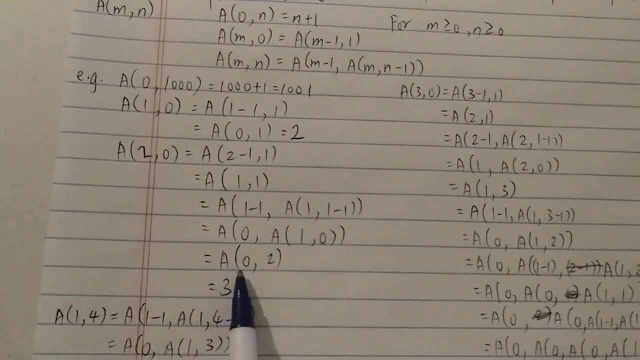 over here. so then it becomes a of 0- 2, because a 1, 0 is. just because this thing it equals to 2, because we already calculate here. if you haven't done that before, you have to solve this one first. so a 0, 2, it equals to 3. 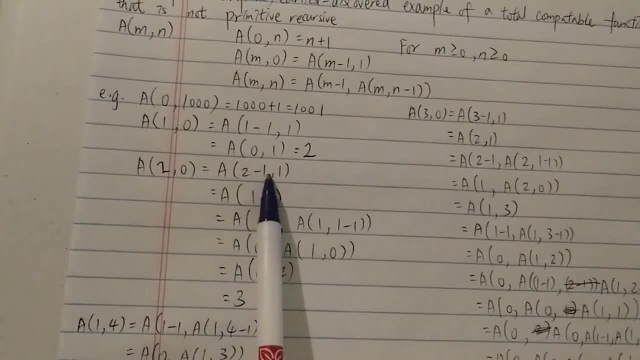 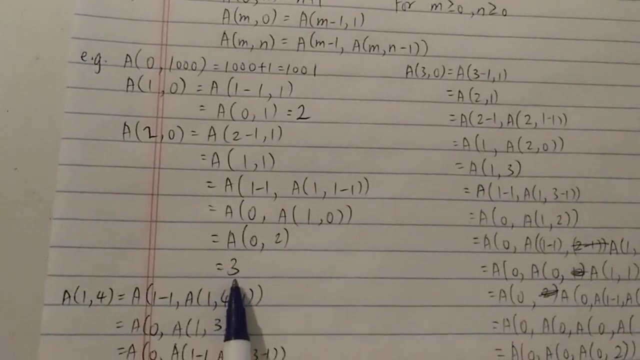 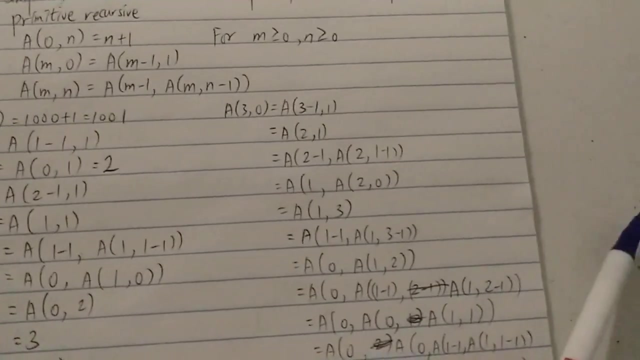 so even a 2, 0, it involves already almost 10 steps already if you count these two as well. but again, you still get a relatively small number. but now what about a 3, 0? so of course you look at the second argument. oh, so it becomes a 3. 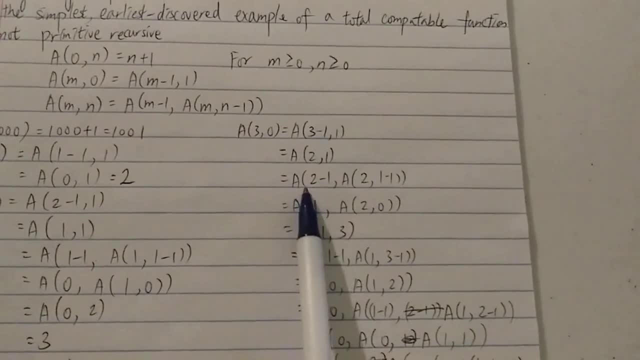 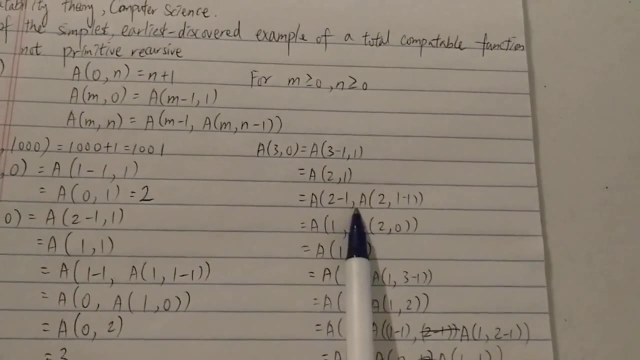 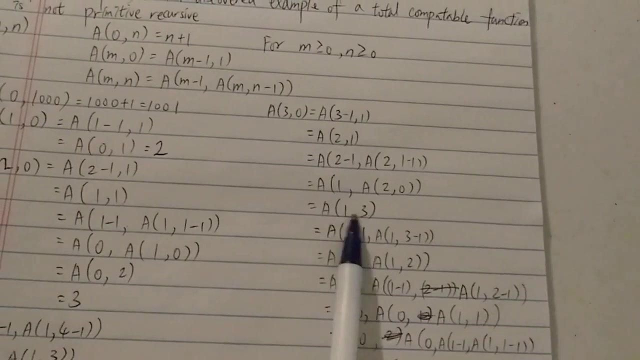 minus 1, 1, which becomes a 2, 1, and then, however, once you get this over here, you have to look at the third argument. so it becomes like that. and then you, and then, however, here you get another non 0, M and M, so you have to look at a third argument. 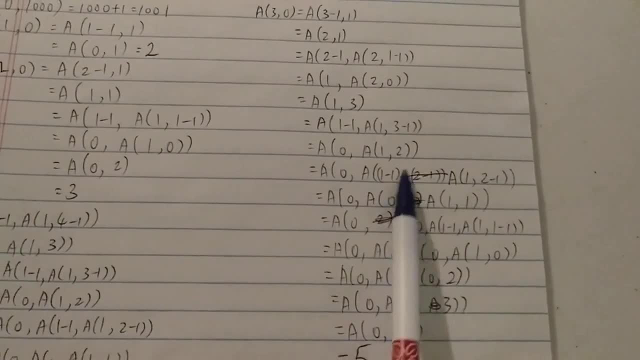 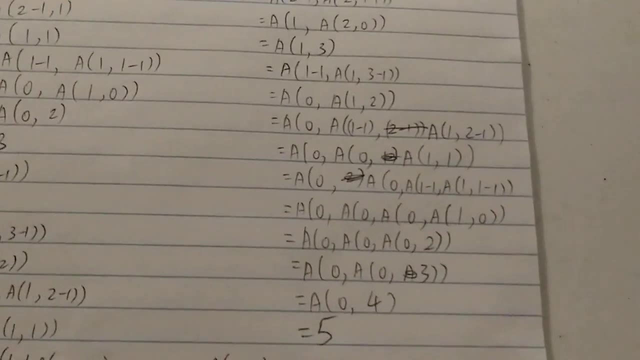 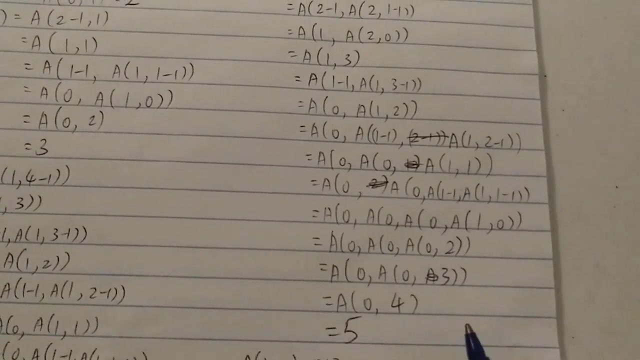 again. so the calculation is pretty long. you know more than 10 steps already, so it becomes this. this is: you can look at it, you can pause the video and calculate yourself or understand yourself, and at the end you get the answer for the five. I mean relatively small answer, but still, if you want to calculate out you. 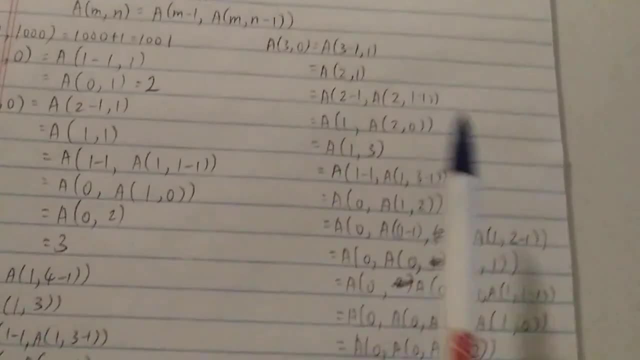 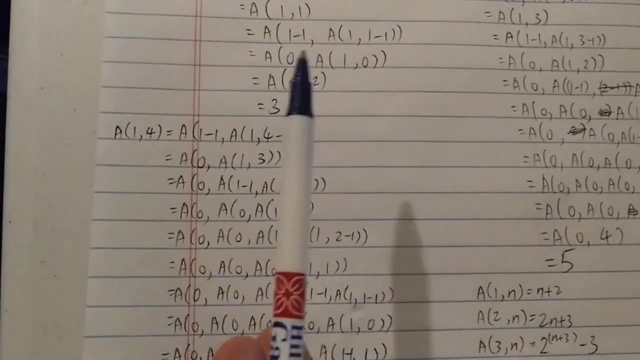 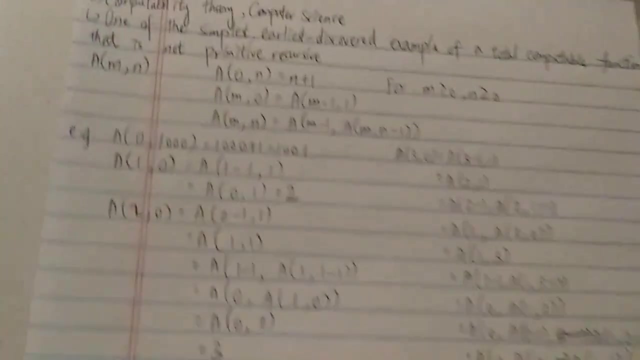 write them all out. it involves even a 3, 0 with a result of 5. you still get a lot of steps. and now let's look at something slightly different. what about a 1, 4? so a 1, 4. of course you look you to start with the third argument over here. so it. 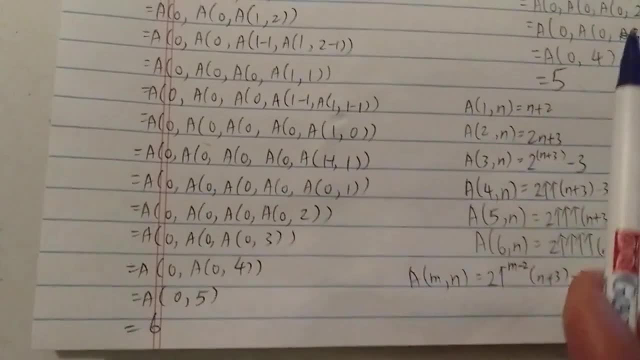 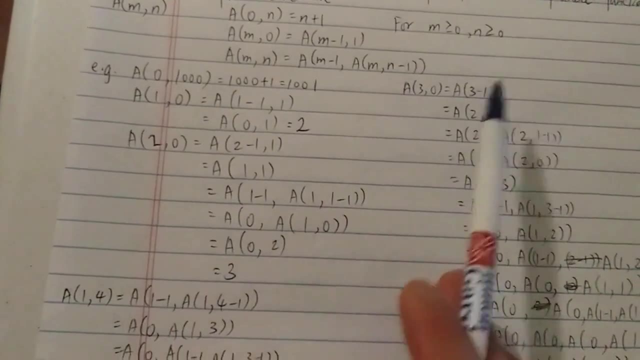 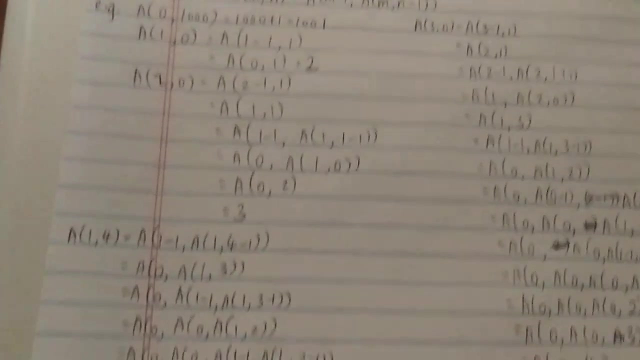 becomes. it looks something like this: it's a lot of steps, because every time if M and N is not 0, you have to bring up the third argument over here, which is, you know, pretty long over here. you have to recall the argument function again. so of course you can pause the video if you. 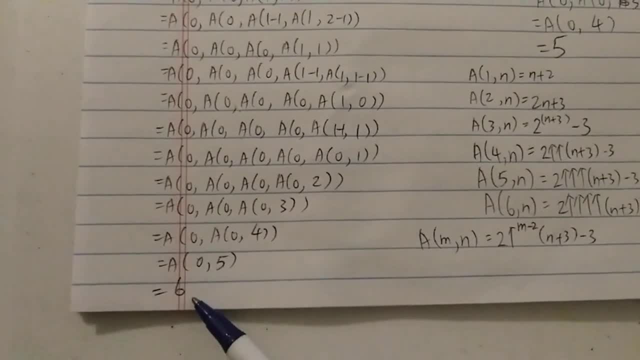 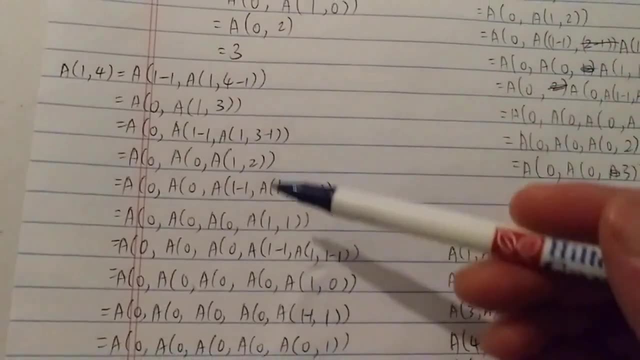 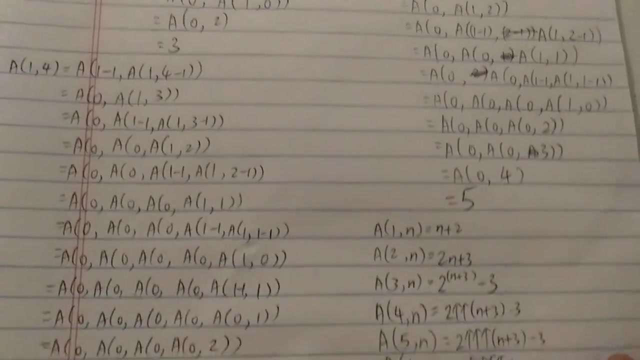 want. it looks something like that, but at the end you get the result of 6. so I mean you can get a very small answer, but you have to do a lot of steps. then remember: 1 and 4 are still relatively small numbers, but I can. I. 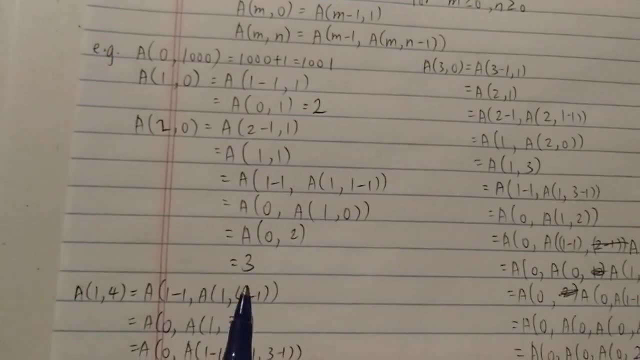 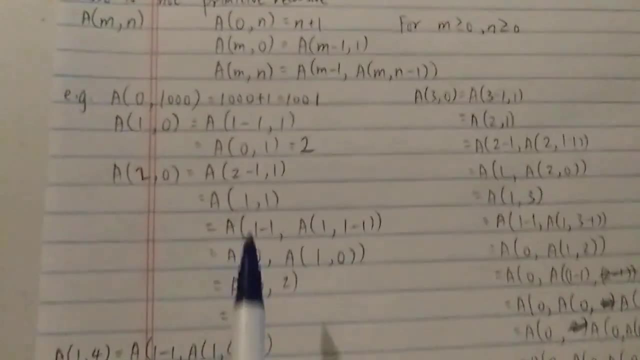 think you already get the idea here. I mean N, I mean M over here is the determinant factor if you have to do a lot of steps and if you get a big answer and of course, as shown over here and doesn't you know, relatively I mean it. 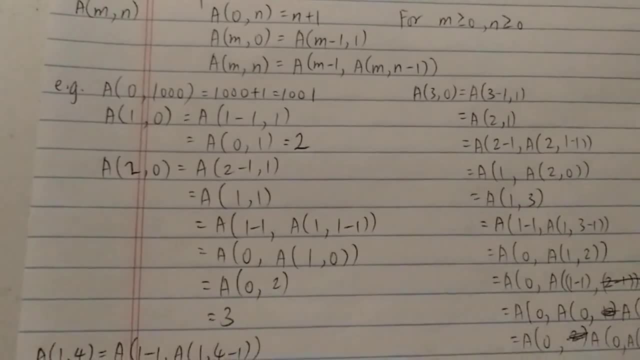 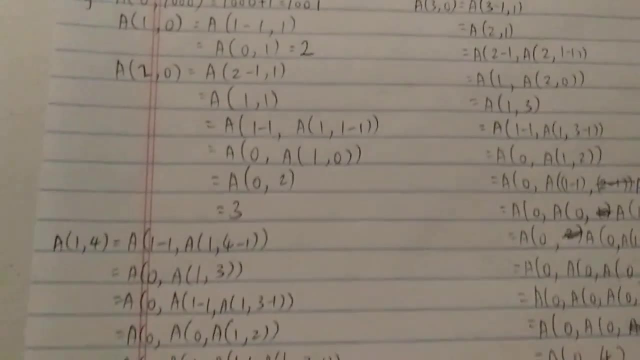 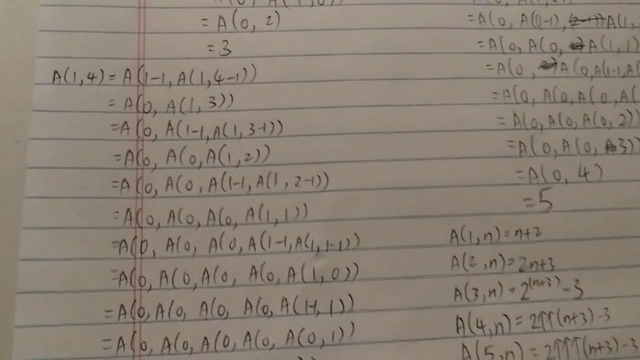 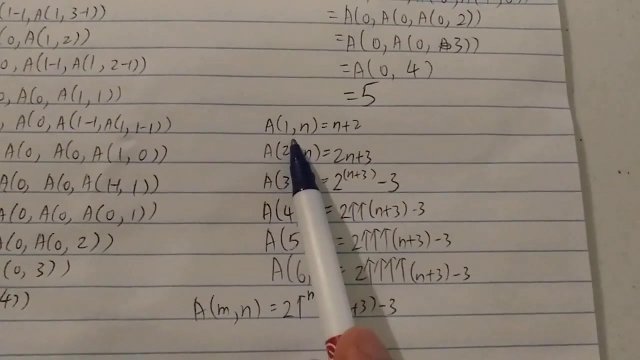 doesn't, is not the determining factor compared with M. you know even N is very big. if M is small, you still. you know it's very straightforward. but if M is getting slightly bigger, as long as M is more bigger than like 2, you really get very complicated calculation. so in general a 1 and it basically, even though 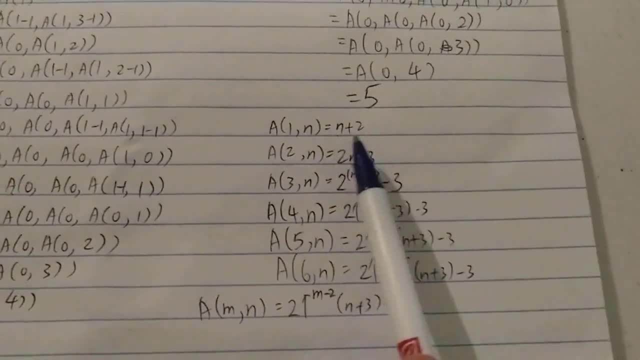 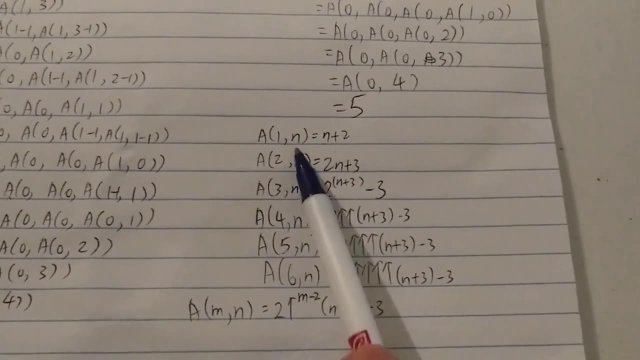 you have to do a lot of steps. basically just equal to n plus 2, but a 2 n. it equals 2 n plus 3 a 3 n. so as you can see, M is increasing over here. then you get 2 to the power of n. 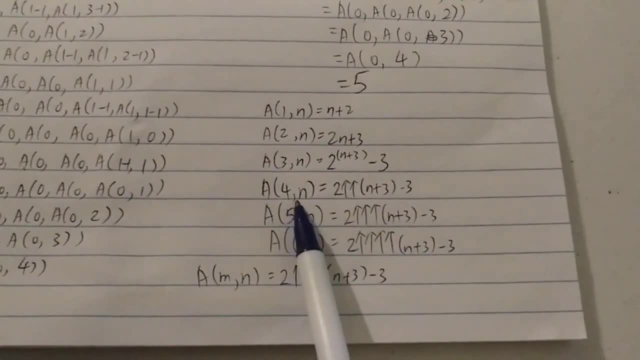 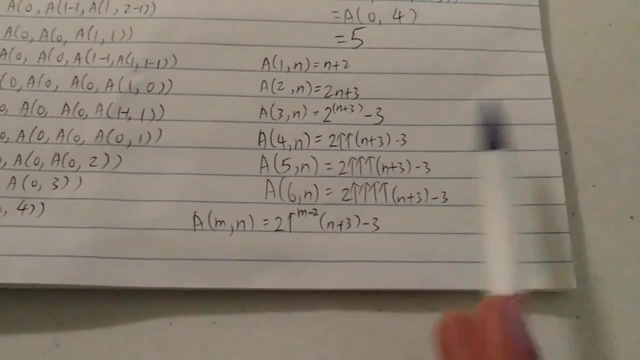 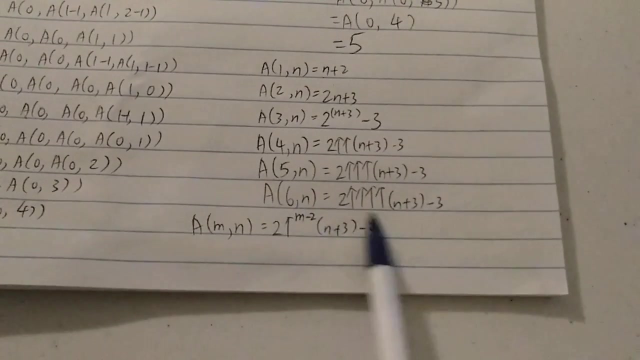 plus 3 minus 3, and then for a of 4 n, then you start. you have to start using the up arrows, or two arrows to two arrows: n plus 3 minus 3. for a 5 n, you see two, I mean three arrows. and then for a 6 n is 4, so you can already see the. 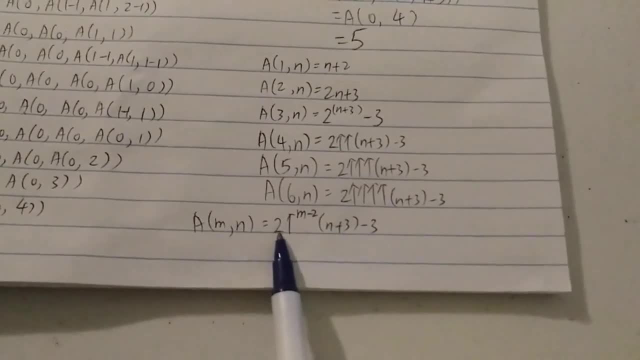 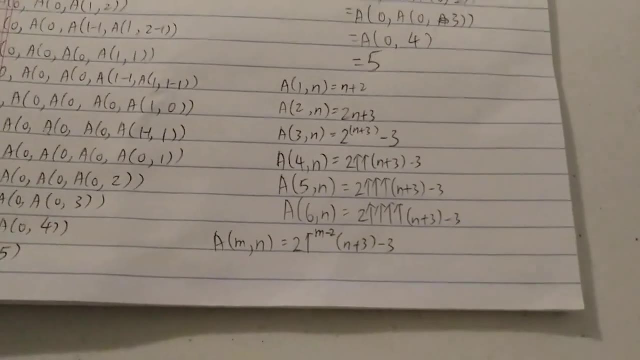 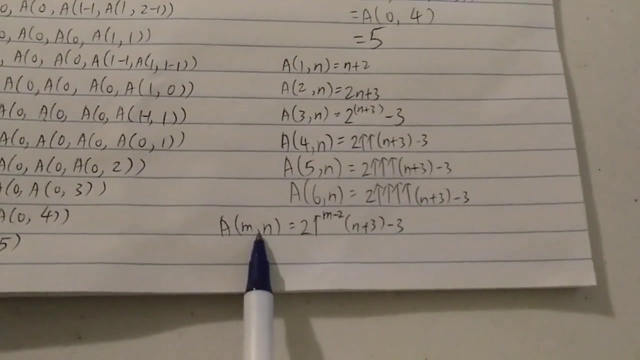 formula over here: a of M, n is equal to 2 with 2, with n minus 2 up arrows, and then n plus 3 minus 3. so you can see, basically M is the determining factor over here. if you get a big M, you know it. 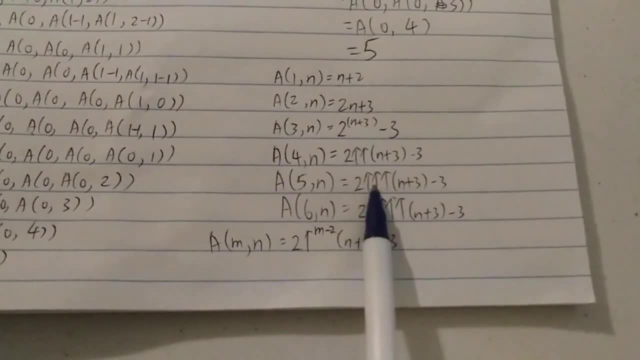 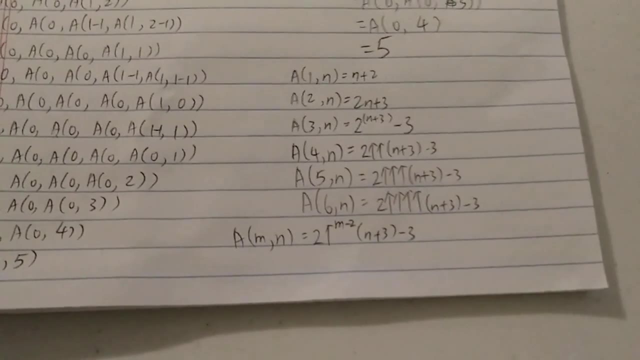 doesn't even have to be very big. let's say 5, then you already you're seeing 3 up arrows over here. if it is 10, then you're getting 8 up arrows. so you're getting big numbers really, really quickly. and let's say: if you get a, 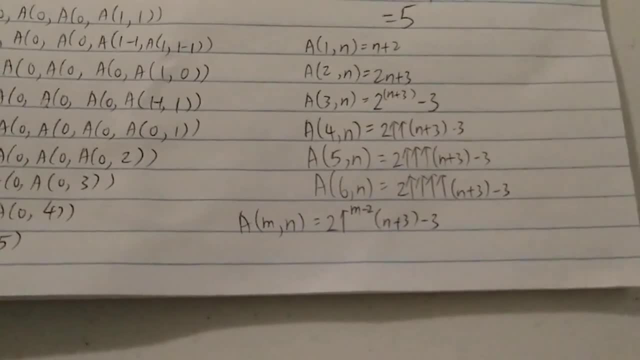 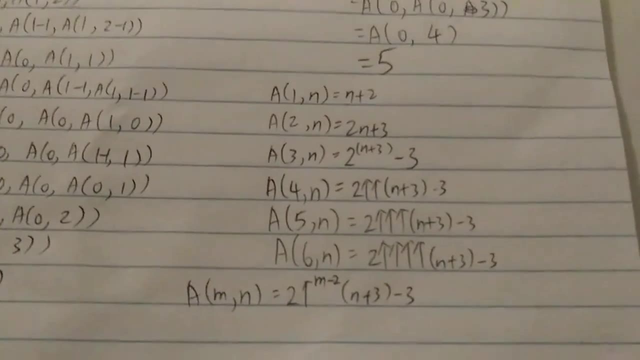 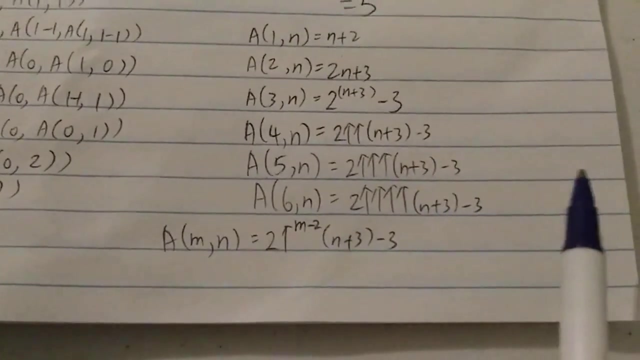 thousand and basically you're getting almost a thousand of arrows. so this is a very, very fast-growing function and of course it involves a lot and a lot of steps. so it's kind of look like the Conway chain arrow notation, but of course that one is even more powerful and you can see. this is why this is a complete recursive.